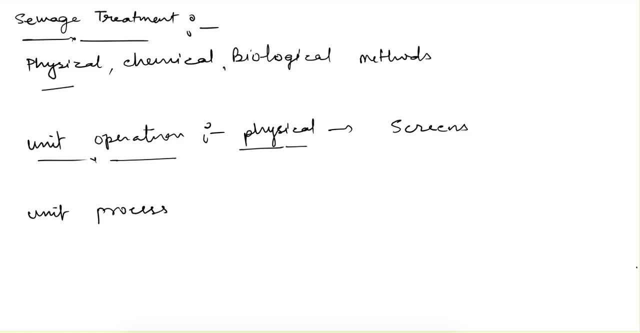 unit operation. we can write some of these. that is, screening. screening will come under your unit operation, then sedimentation grid chamber. these are all your unit operations, Whereas if chemical or biological forces are applied, chemical, biological methods are applied for the removal of impurities. 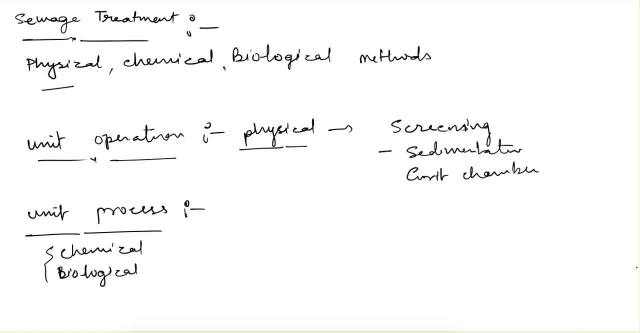 impurities such as organic matter, then we term that particular method of treatment as unit process. so the various methods that some of them we'll write here so that come under here are: oxidation pond, then you can take trickling filter, activated sludge process. these are examples of unit processes. that is your basic classification. 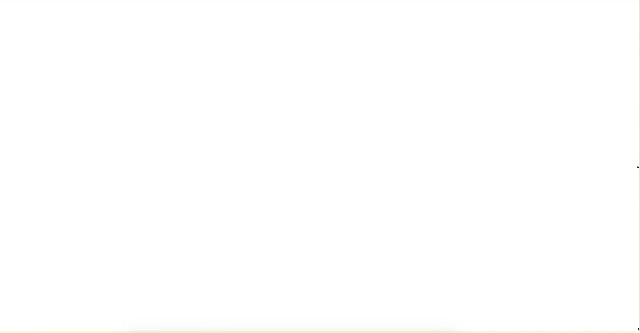 then we can see what are the various steps in which treatment is given to sewage. so initially there is preliminary treatment, preliminary treatment. so preliminary treatment, preliminary treatment, is done to remove floating, floating impurities or floating materials. we can write, apart from that some inorganic, suddenly both solids. 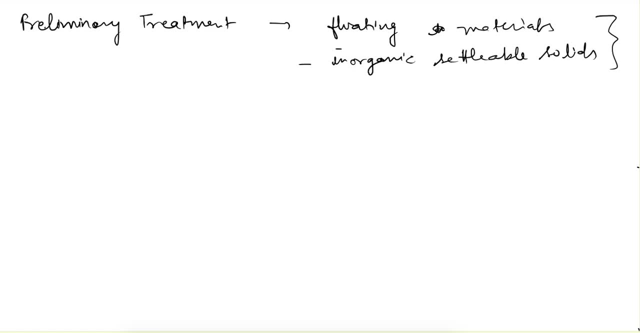 so what are thethese are removed in your preliminary treatment so that the further load on the treatment plan will be reduced if we remove them. that is, floating material materials as well asН such as your wood can be there, or some paper or some resettlable solids like metal and 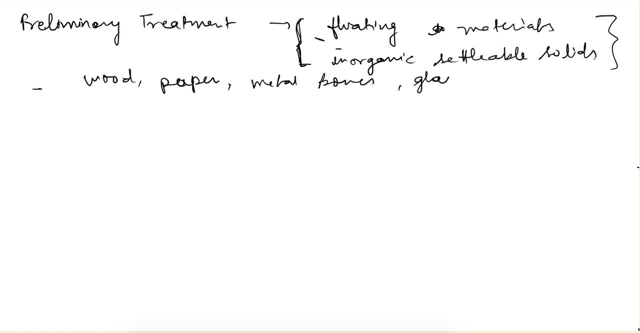 bones can be there, glass can be there. all these will be removed in your preliminary treatment. So the treatment that come under this one, that is, screens or grid chambers- that is basically here we are applying unit operations or the physical forces- are predominant in case of preliminary treatment. that's how you can remember it- skimming tank also. so these are all your. 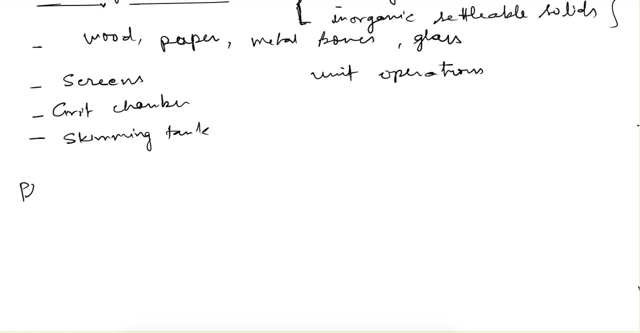 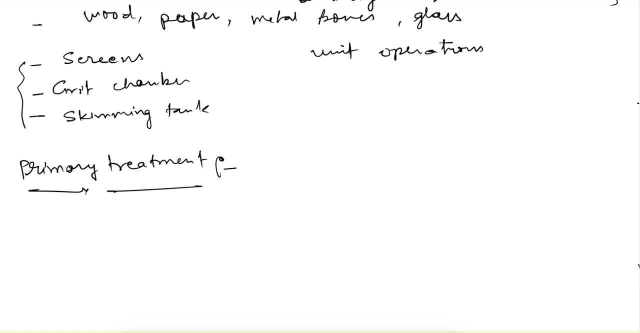 preliminary treatment methods. after that next step would be primary treatment. so sometimes whatever we have covered in preliminary treatment, These methods are termed as preliminary treatment. These methods are termed under primary treatment also. so you should not confuse. I mean preliminary and primary treatment. both are both depend upon these unit operations, that is, physical. 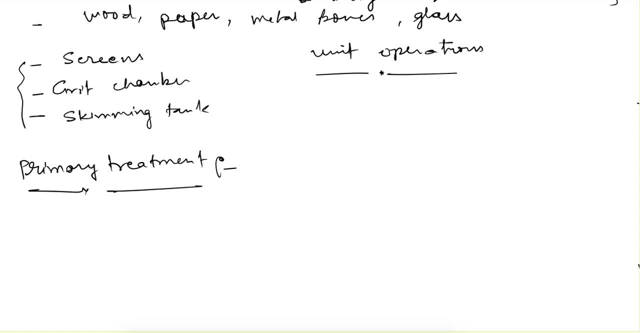 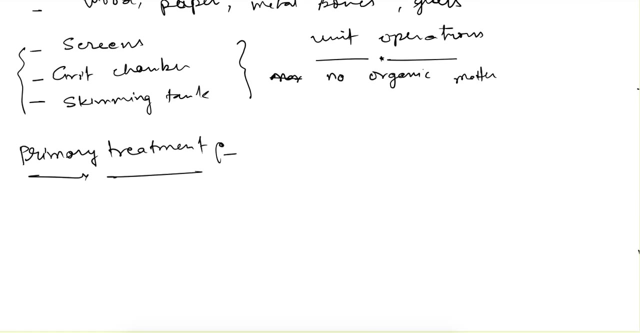 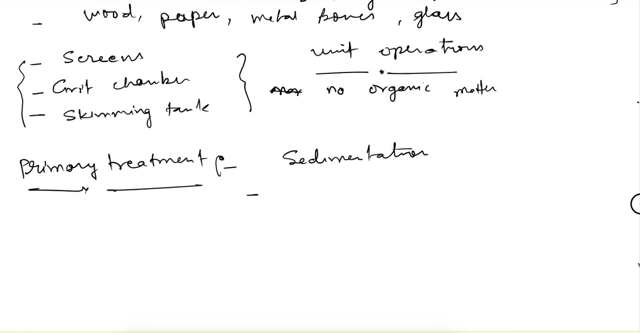 forces are predominant in case of, in case of preliminary treatment. you can remember one thing that is: here no organic solids are removed, no organic matter, whereas in case of primary treatment, One of the example is sedimentation. so this sedimentation, if preliminary treatment is given, then your inorganic settlable solids will be removed in preliminary treatment. such 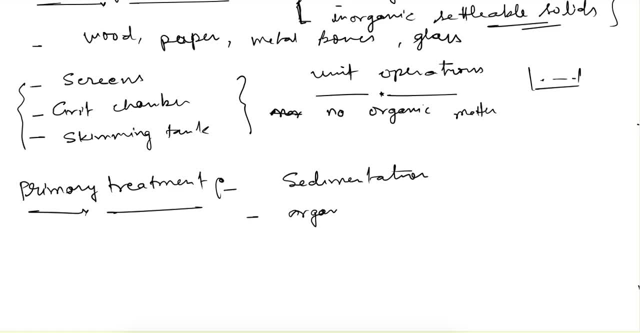 as grid chamber, whereas organic solids will be removed. I mean not all the organic solids, but some of them will be removed in primary sedimentation. so around 60 to 70% of suspended solids Are removed in this Primary sedimentation, and that is your, that is your primary treatment. so, whatever solids, 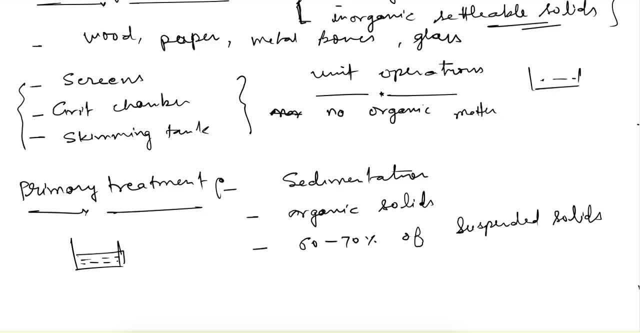 are removed here, so these will be organic solids, if we have given preliminary treatment. so these settled solids have to be sent to a sludge digestion tank so that this organic matter can be stabilized. This we can see later. also just to give you a brief idea. and if preliminary treatment 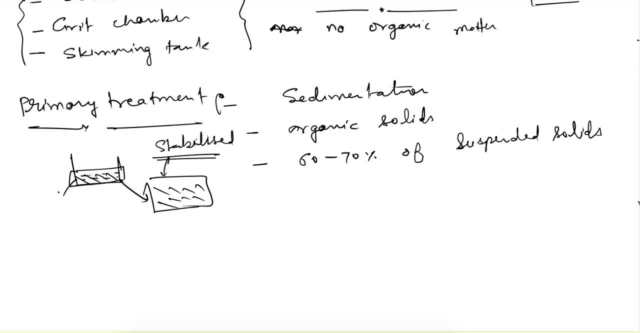 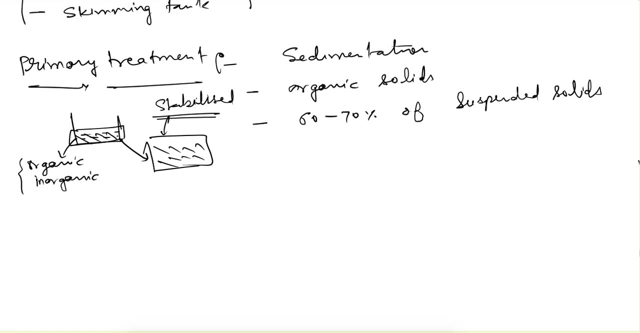 is not given. In this primary sedimentation both organic as well as inorganic, inorganic, inorganic particles will settle, but it is not preferable because it will increase the load on these sludge sludge digestion unit. After that preliminary treatment we have, I mean so primary treatment- we have secondary. 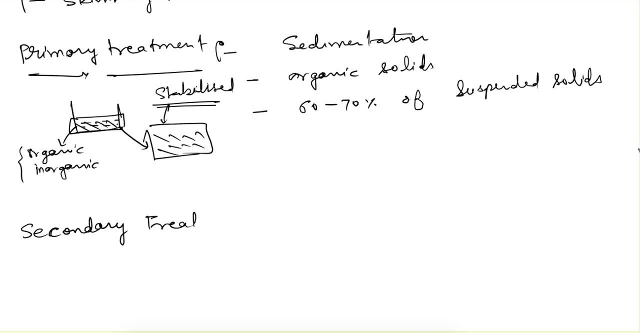 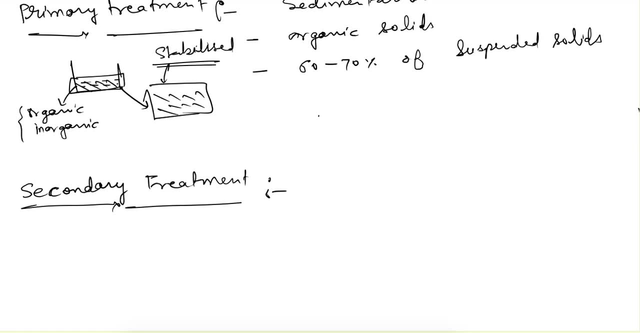 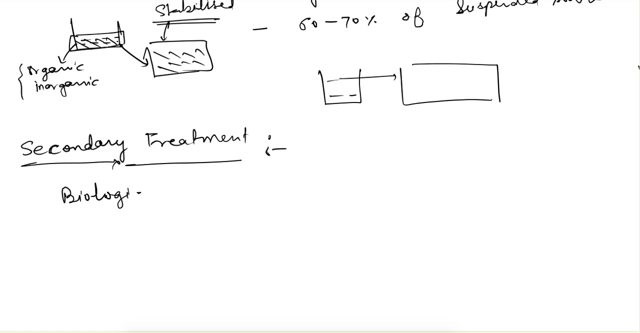 treatment. So That is after primary treatment. whatever sewage we get, that will be sent to next unit. and these are. these come under your secondary treatment units. so in these units mostly biological treatment is given, That is, it is done by the active Microbial. 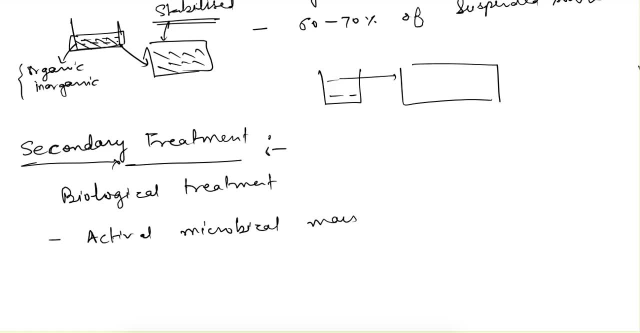 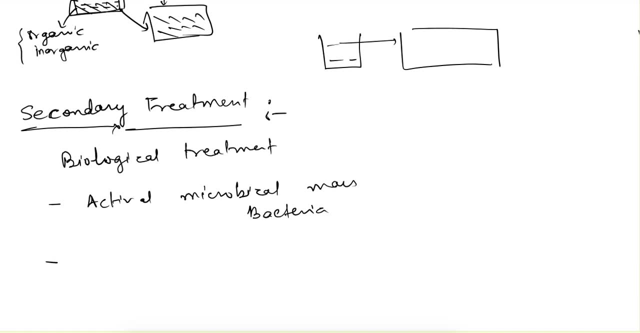 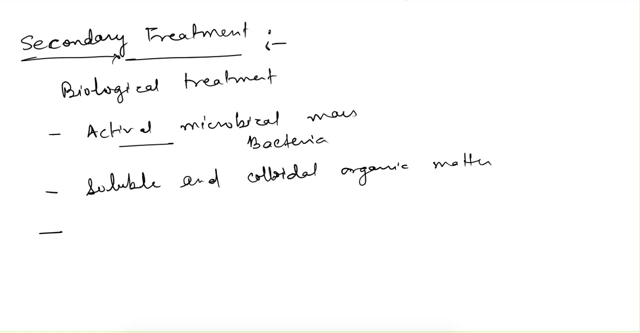 Mass, Or we can say Microbial Bacteria. So the methods, I mean what is removed here, so soluble, Soluble and colloidal organic matter. Colloidal organic matter: these will be removed in your secondary treatment units. So, as I said, it contains a large amount of active microbial bacteria. 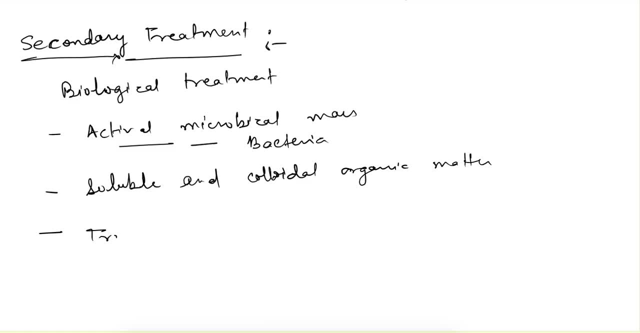 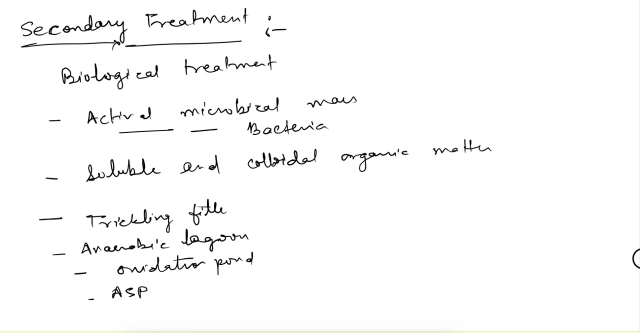 And what are the processes or the methods? So trickling filter and your anaerobic lagoon, as well as oxidation pond, or you can take ASP, that is, activated sludge process. these all come under secondary treatment, so most of the treatment plants are given. 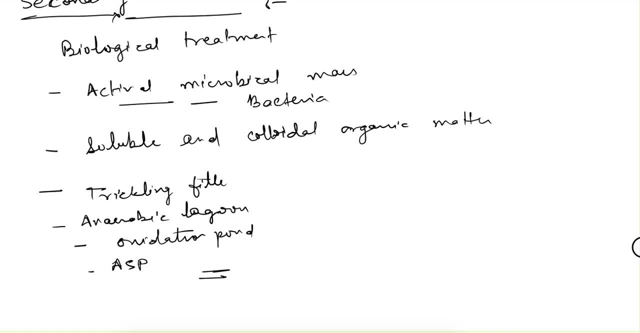 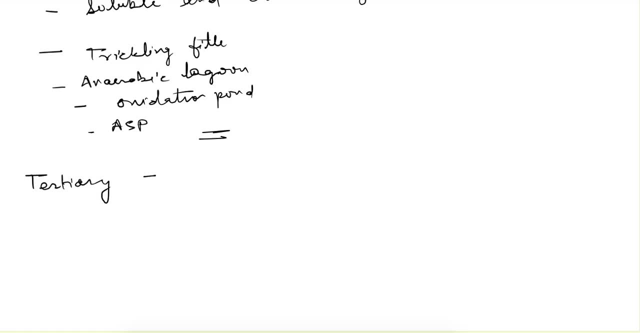 I mean They give the treatment up to this stage, but in some other cases Last stage, that is, tertiary treatment, It is also given. So it is mostly used when, When there are- I mean some of the you know inorganic impurities such as. 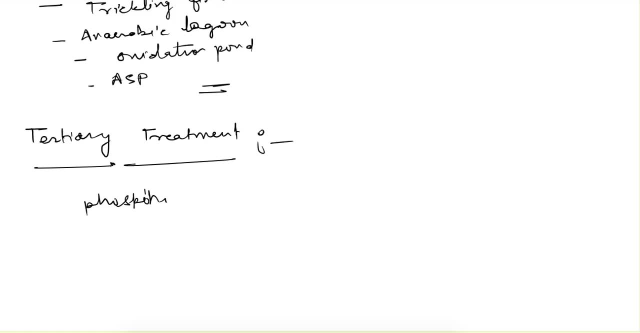 Phosphorus, Phosphorus, Phosphorus. Phosphorus has to be removed and nitrogen has to be removed, because if we leave the water with phosphorus and nitrogen in some stream, then it accelerates the growth of algae. So it is preferable in some cases to remove these. these also. I mean these are inorganic. matters. So for that, denitrification has to be done And apart from that, apart from that, tertiary treatment is given When this water, which we are releasing from this wastewater treatment plant after just after this point, it has to be again collected for drinking water treatment. 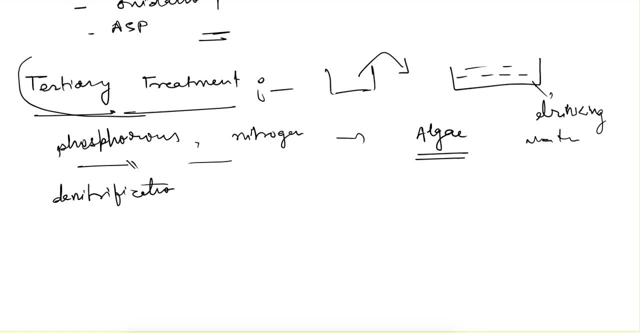 Drinking water purposes, then that waste has to be necessarily given this tertiary treatment. So in that case some other methods which are used, so activated, I mean adsorption with activated carbon, This, This, This can also be given as a treatment and disinfection can also be done. 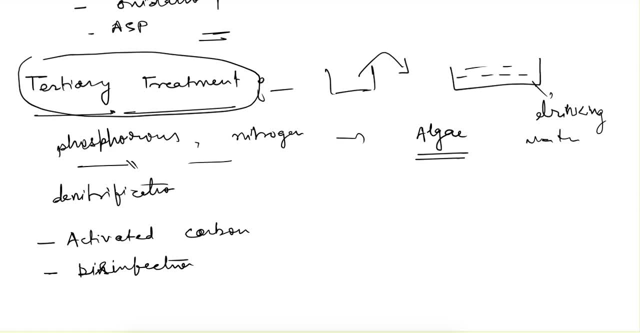 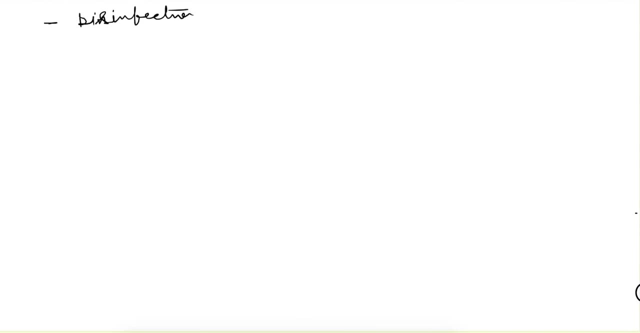 Disinfection to kill the pathogens, because further we are going to use- I mean- similar sources for the drinking water purposes, So disinfection has to be given. So these are the processes. I mean a brief overview of the processes that are used in case of sewage treatment. 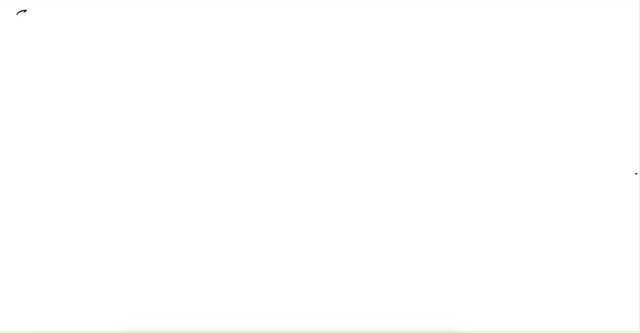 So now let's see, For example, about these, for this sedimentation, Different types of settling. are there types of settling? So I will not take complete all these great chamber and primary sedimentation, because theory is similar to what we have already seen in water treatment. 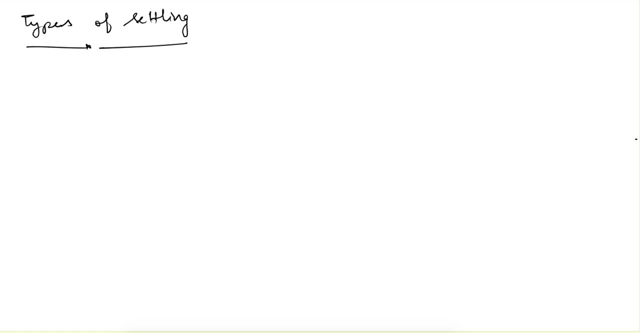 So I'll just cover, and after this we do, we start with trickling filter and then activated sludge process And later whatever is necessary that we can cover. So these different types of settling are there in case of sedimentation that we can see here. 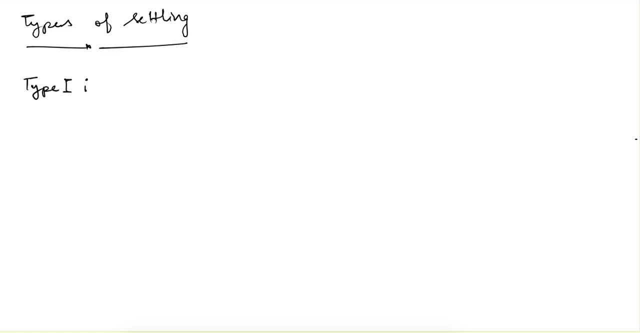 in brief, that is type 1, type 2, type 3 and type 4 settling. So type 1 is your discrete settling. Discrete settling means what we have seen in plain sedimentation, that is, there are no inter particle forces. So 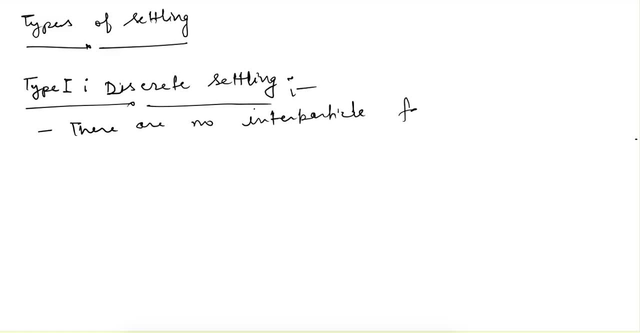 So, Or we can say: a particle and all the particles, all the particles are settling freely. So that is. it will happen in case of if sand is there and grit is there. So these settle very easily without the, without causing any hindrance to other particles, and 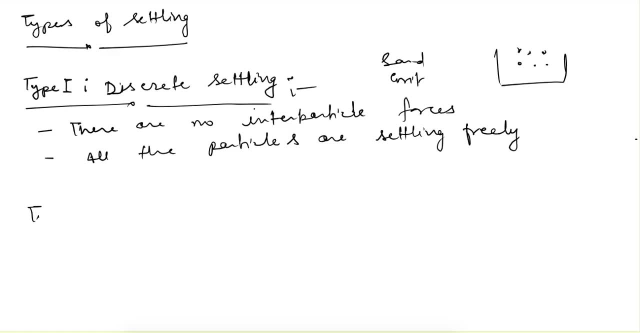 that come under your type 1 settling And you have type 2 settling which is known as flocculent settling. So flocculants in flocculent settling. you can obviously understand with the name also. So these flocks will form. initially we have these colloidal particles, but they form the 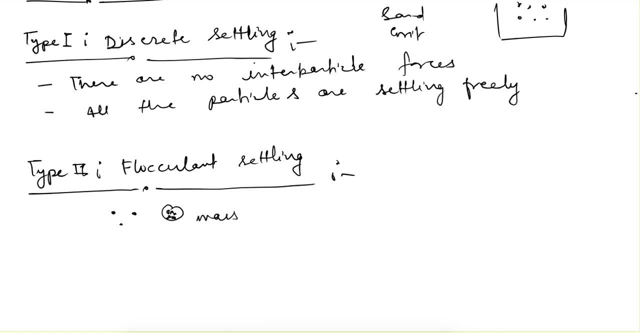 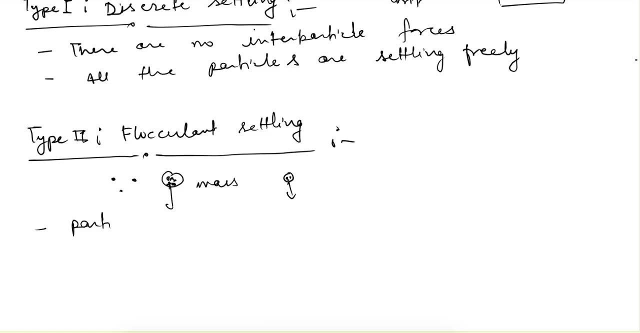 flock and so their mass will increase and then they will settle at a very high rate or with a very high velocity. But here some inter particle forces are working, you can see. So particles form flocks to settle And then these, due to formation of these flocks, this mass will be more so, this settling velocity. 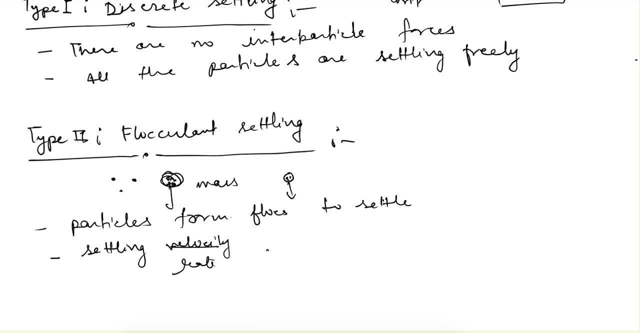 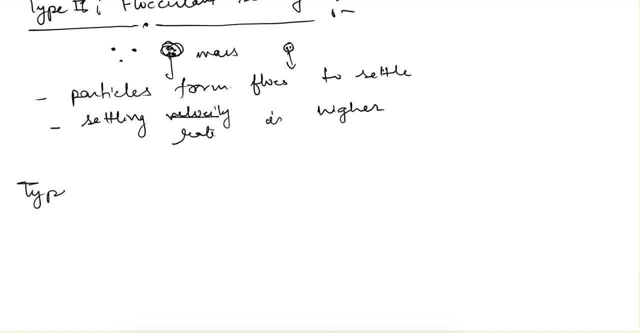 settling rate is higher. settling rate is higher, So So This is your type 2 settling, then we have type 3 settling and that is your hindered All zone settling. So flocculation, I mean flock formation. it happens because we have already seen, when we 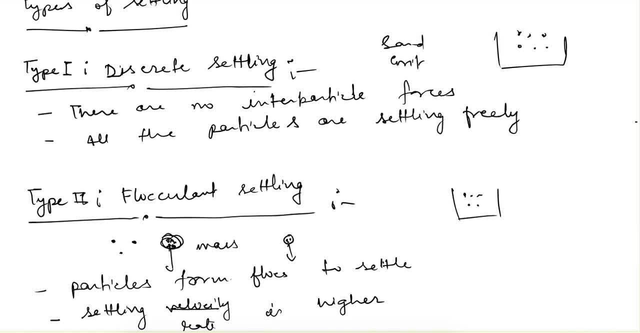 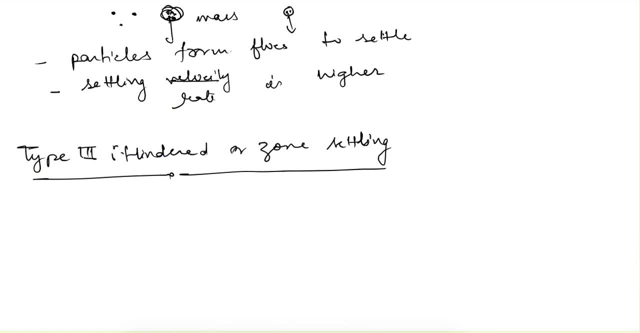 add some coagulant. this, This discrete settling, will happen if we have these bigger particles like sand and grit. and after that, in case of secondary sedimentation tank, what happens in the lower zone of the sedimentation tank? these between these flocs also, or particles also, inter particle forces act. So this is one floc or one particle. 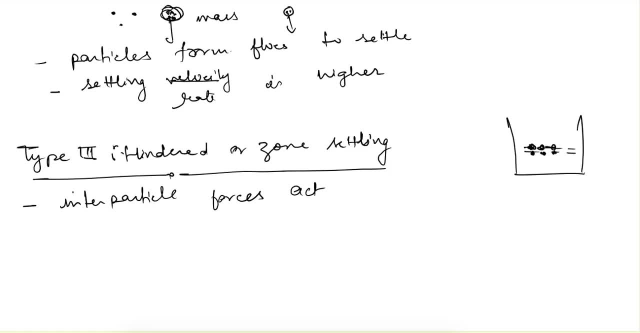 and another point: we have another particle, So some inter particles forces will be acting so that the relative position of these particles they do not change. I mean they will settle as a whole bigger mass, So this whole unit will be settling together. It will happen like that because some inter particle forces are acting. 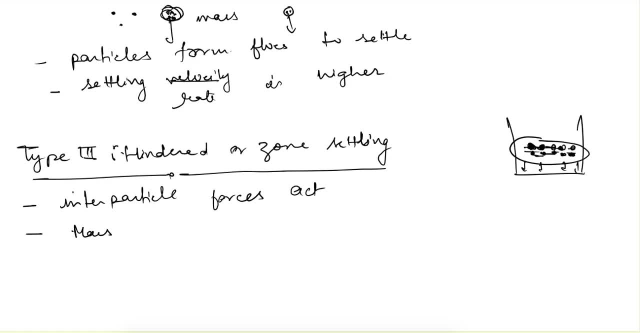 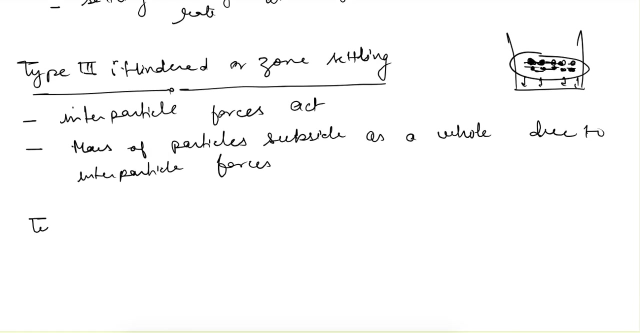 So you can see. I mean we can write mass of particles subside as a whole due to inter particle forces. Then you have the last one, that is, type 4 settling, which happens in the lowest zone, lowest part of a secondary sedimentation tank. we can write for type 4 settling, which is known as: 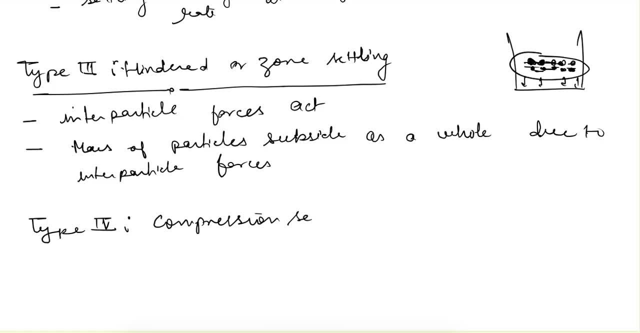 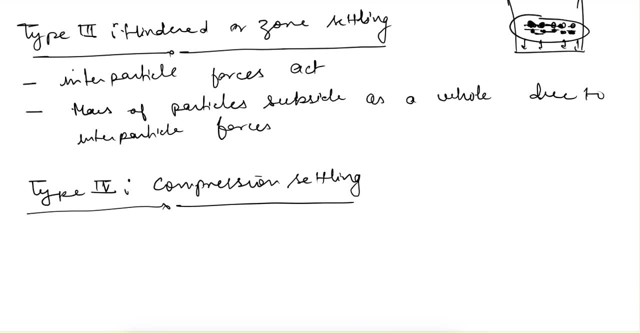 comfort zone, Compression, settling. So as we go below this hindered zone or zone settling in this lower part, these particles will come in contact with each other and they will form a structure. They are in contact with each other and they will have some pores in between. So a structure is formed, Structure is formed and any further settling can. 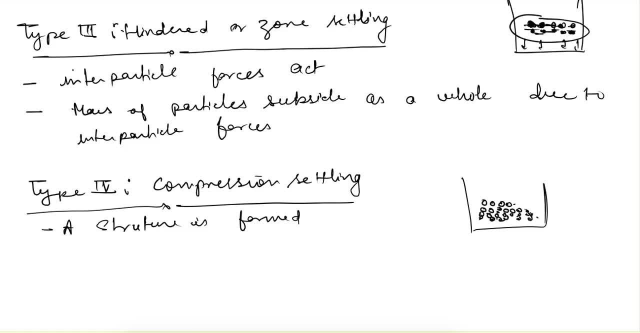 only be done when you are adding some more mass of particles, And that is obviously happening. more particles will be coming down and it will add to the. I mean it will increase the load on this structure. So because of this increased load, further settling will be happening. That is your type 4 settling. 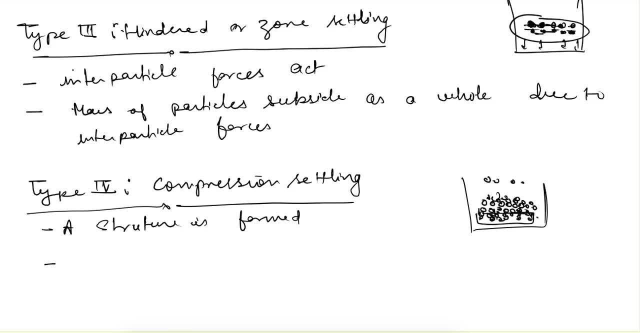 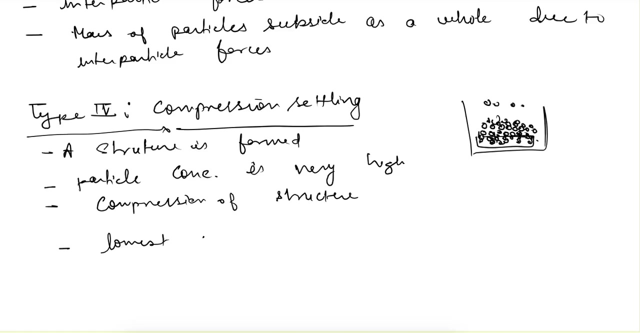 So it forms a structure and in this zone particle concentration is very high and the further settling happens due to only compression of structure. So, as already I have told, this happens in the lowest part of secondary or 2 degree sedimentation tank. So, as already I have told, this happens in the lowest part of secondary or 2 degree sedimentation tank. 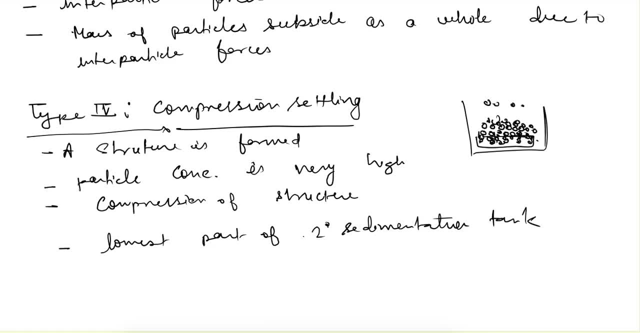 So, as already I have told, this happens in the lowest part of secondary or 2 degree sedimentation tank And apart from that, in sludge digestion tank also it happens. So this is just a brief overview about different treatment methods and about these settling zones. Now, after this, we will start with the more important topics, that is, your trickling filter and activated sludge process. Thank you,